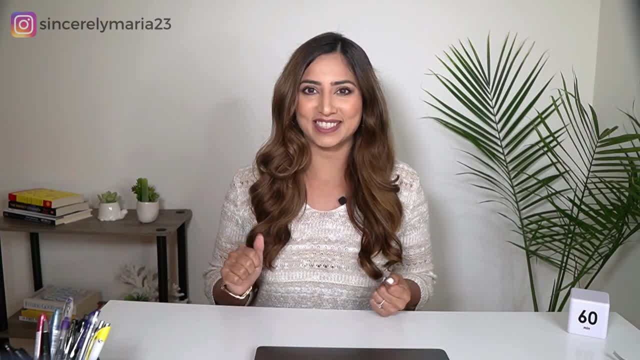 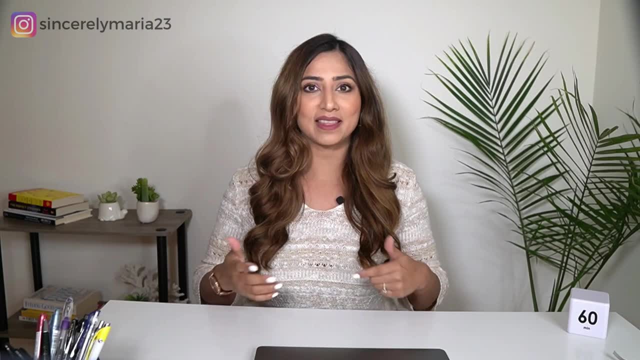 from today's video. I will walk you through five exercises so you can start implementing them right away. You don't need to do all five. Pick the ones that work the best for you and that you can incorporate into your schedule. But if you can do all five, then I do guarantee. 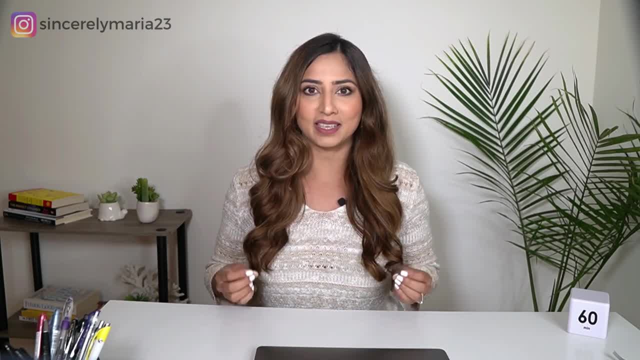 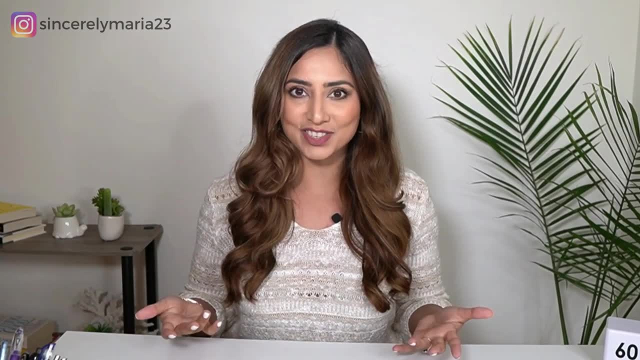 that you will start to see massive changes in your speaking abilities right away. But first, if you are a professional who wants to improve your public speaking skills, your presentation skills, or just be able to sound more confident when you speak, then do subscribe. 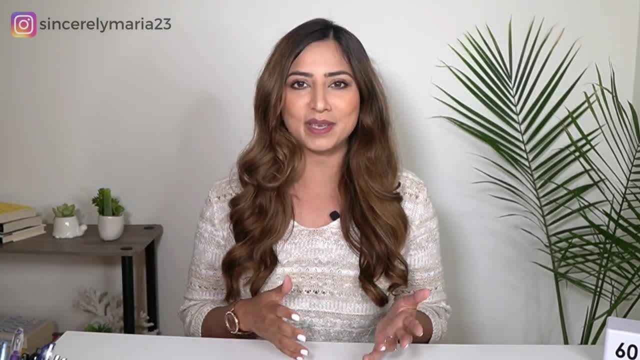 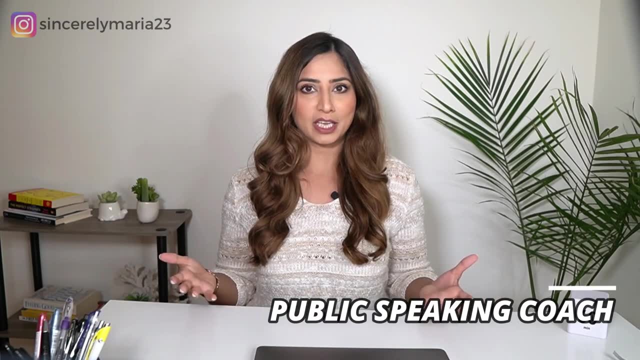 to my channel because I post videos and resources to help you become a more confident speaker. Also, if we have not met yet, hi, my name is Maria Malik. I'm a public speaking coach. I run an online program called the Speak With Confidence Academy, So the academy helps people go from being 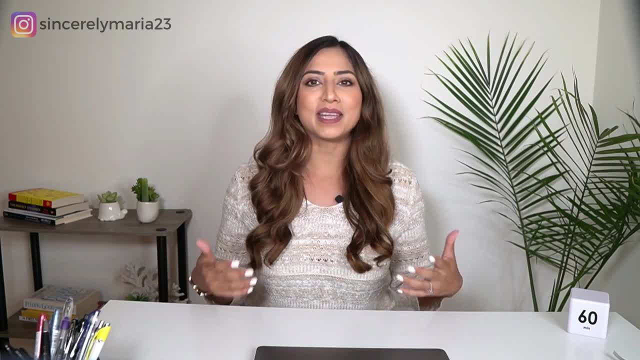 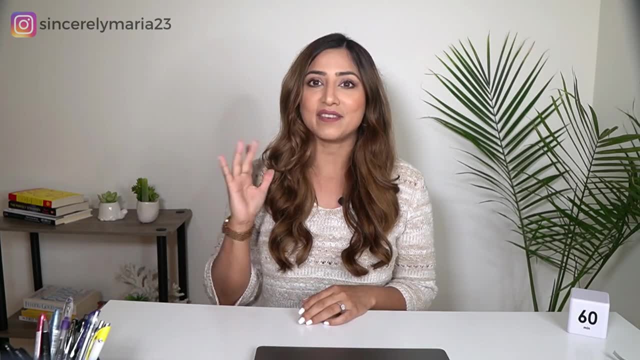 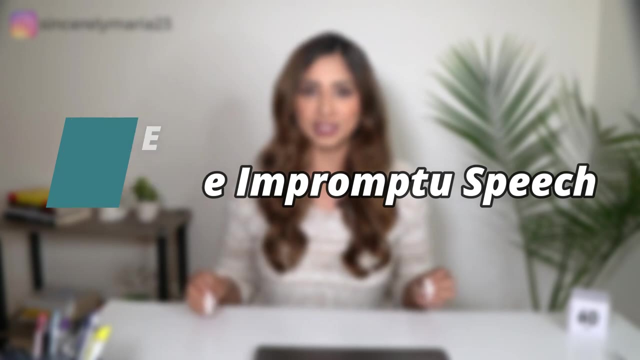 shy, nervous, afraid of public speaking, to becoming enigmatic, confident speakers who really leave an impact on their audience. Let's get started on the five daily public speaking exercises. Exercise one practice: impromptu speech. Impromptu speech is when you have to get up and talk in front of an audience. 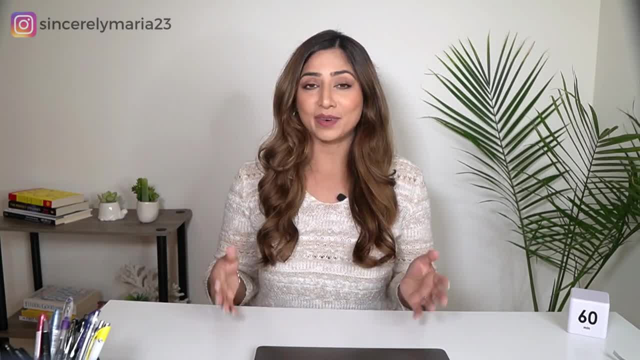 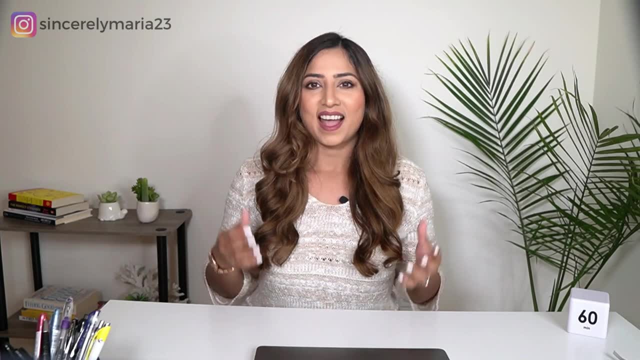 about a topic that you have not already prepared for. I run this exercise with my clients weekly and they love it. It's also one of the places that they see the most growth. I am leaving a link to the impromptu speech questions that you can use to make it a little bit easier for you. 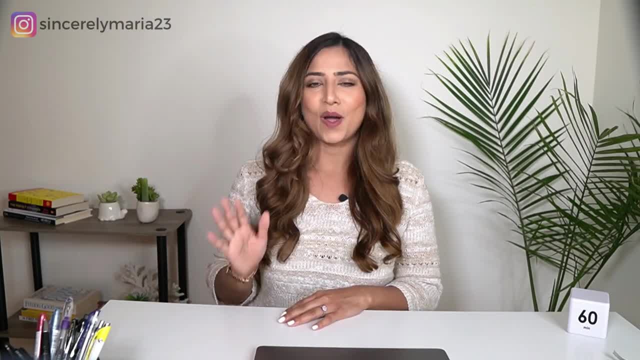 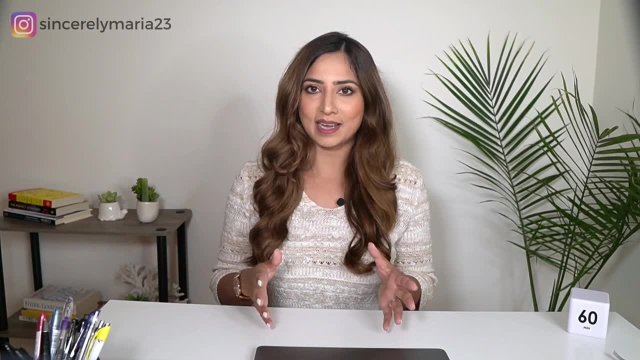 There are more than a hundred, so you won't run out anytime soon. All you have to do is, once a day, pick one question and answer it. If you have any questions, please let me know in the comments And answer it out loud. For example, the question can be: explain how a smart person cannot be wise. 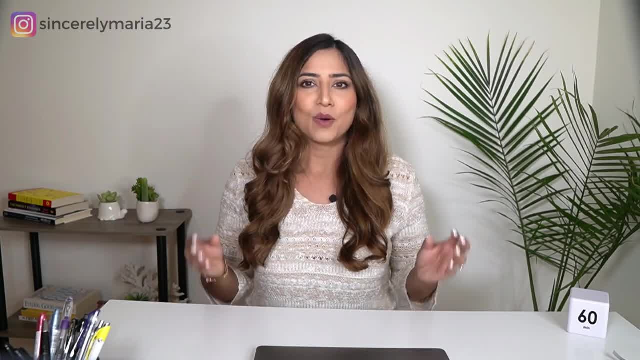 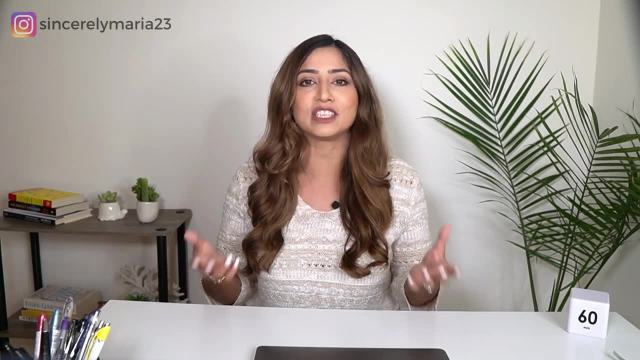 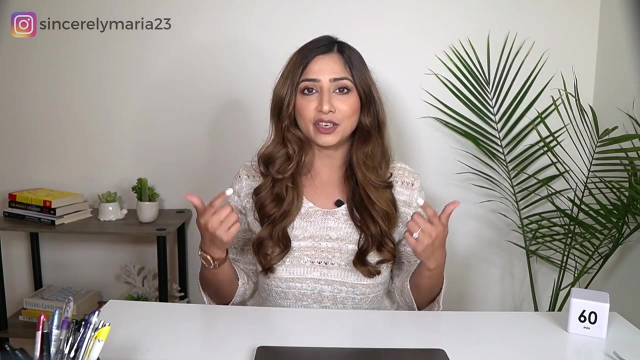 or who was your role model and why? One of my favorite questions to ask my client is: what is the first thing that you would do if you woke up in the middle of the jungle? The point of this exercise is to get you thinking and formulating well-structured answers in your head really fast. 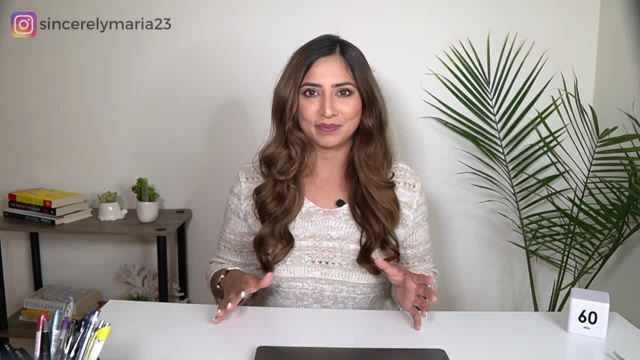 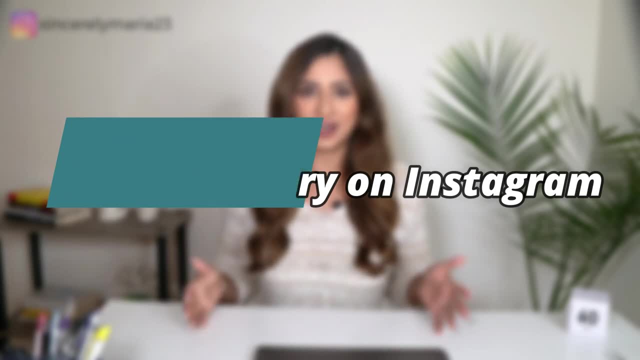 This will, in turn, help you become a better speaker. So if you have any questions, please let me know in the comments And you'll be ready the next time you're put on the spot. Number two: create a story on Instagram So, before you run away, remember you don't have to post it. 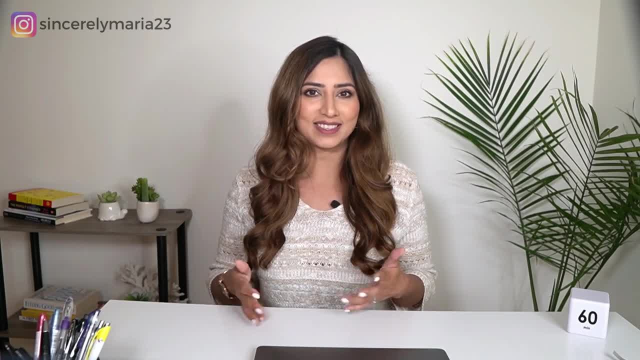 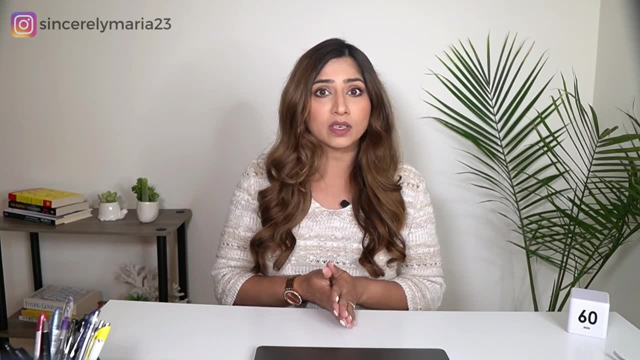 I also love this one because it also helped me get over my camera shyness. So once a day, grab your phone, open up stories on Instagram and talk about your plan for the day or something that happened to you recently. that's interesting. You don't have to post it if you don't want to You. 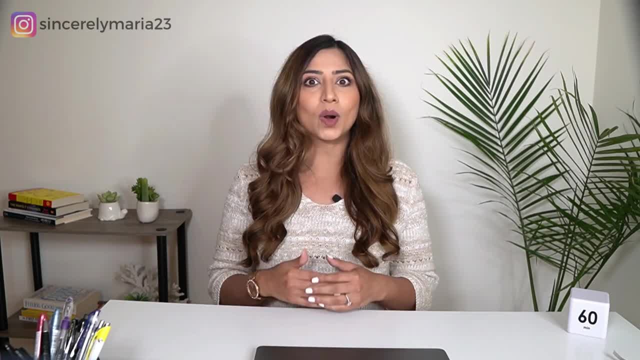 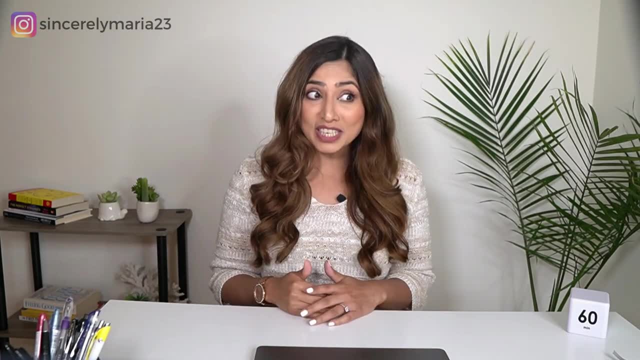 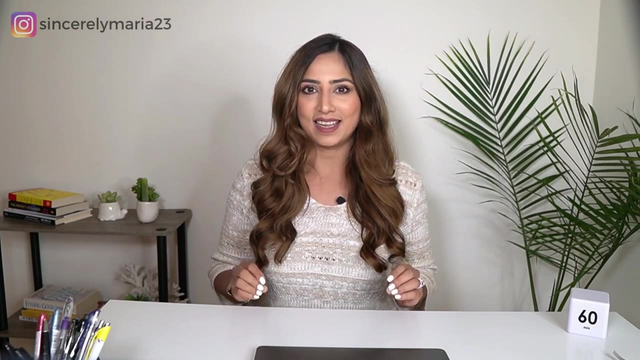 can, if you feel comfortable with it, After posting it or saving the video, go back and watch it as many times as you can. If you cringe, it's okay, but you will know what not to do next time and you will continuously get better each day. If you do post it, tag me on Instagram at sincerelymaria23. I. 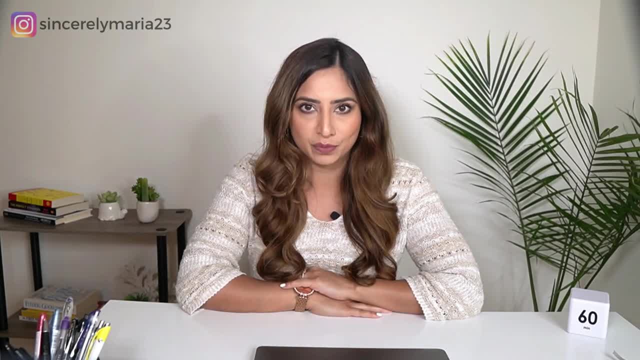 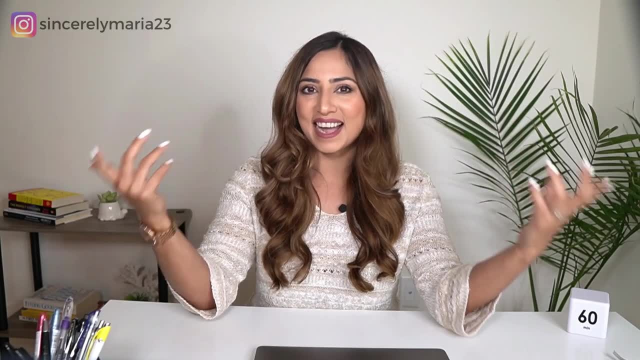 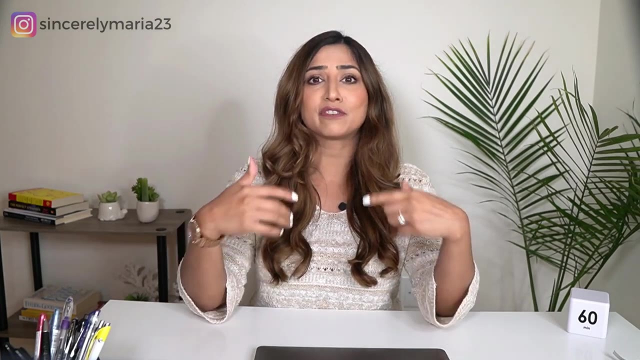 would love to see your progress. So number three of the daily public speaking exercises is to do enunciation Practice. If you have taken acting classes or drama classes, then you already know what these are. In case you don't, enunciation exercises help you differentiate your vowel sounds and 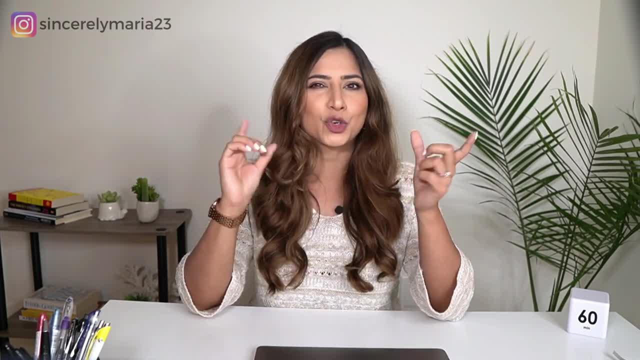 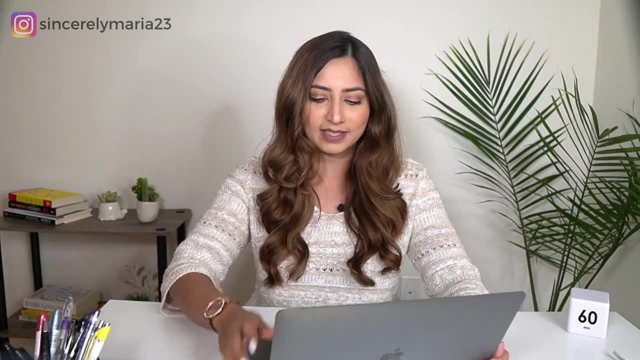 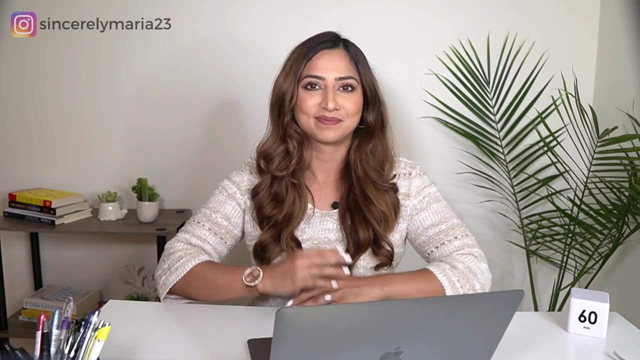 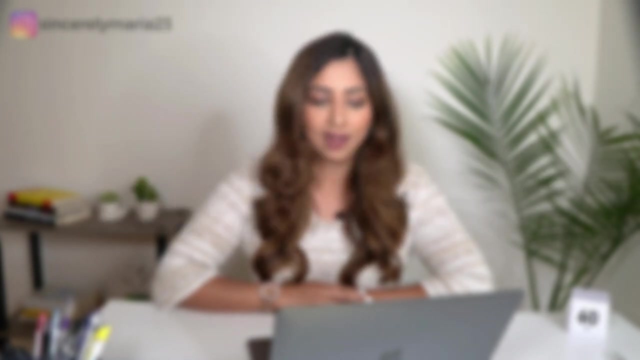 make the beginning and end of each word very distinct and crisp. This is basically training your mouth to sound more clear. Actually, let me give you an example of an enunciation exercise. Here found one: Four furious friends fought for the phone. Fine white vinegar with veal Five. 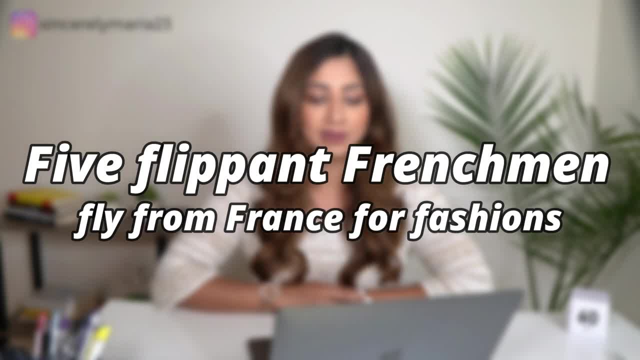 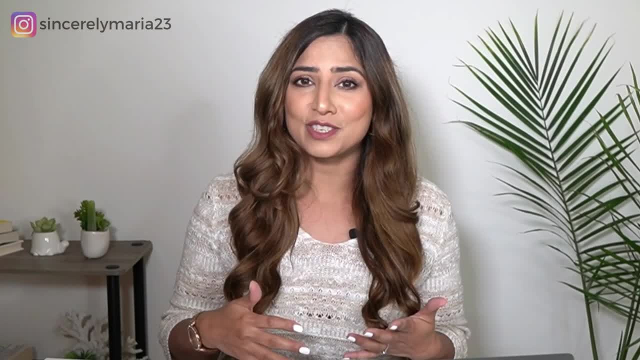 flippin' Frenchmen fly from France for fashions. Five flippin' Frenchmen fly from France for fashions. The free thug set three thugs free. These are honestly so fun to do, and any time that I have to speak or do a presentation in front of an audience, I always do an enunciation exercise. 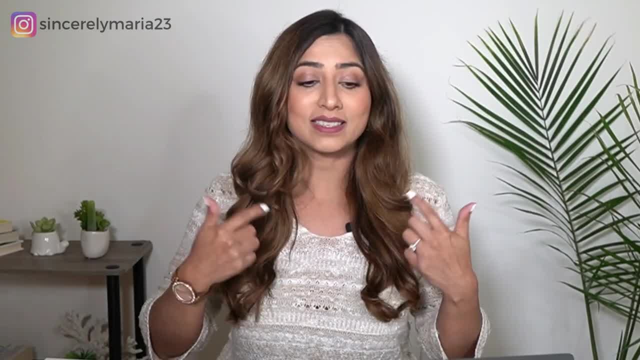 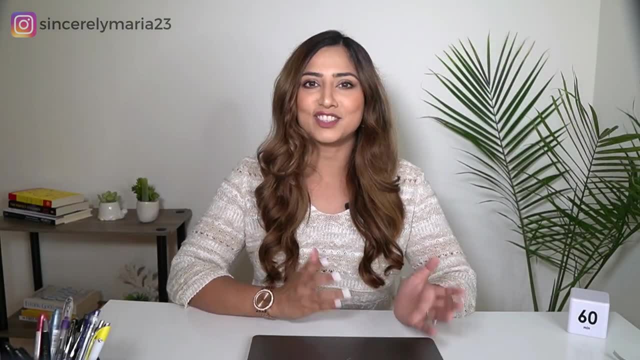 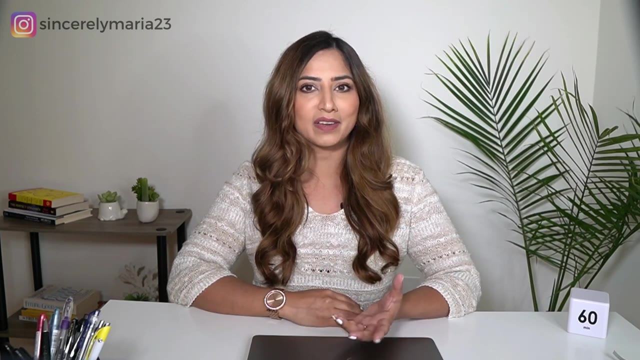 I always do a few of these just to get me into the rhythm and avoid stumbling over words. Let me put this away. There are so many of these online. Just google enunciation exercises and you will find a whole bunch. I will also leave a link to some of my favorites down below, just to save. 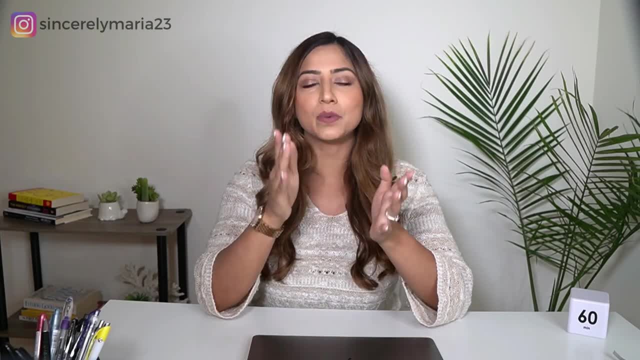 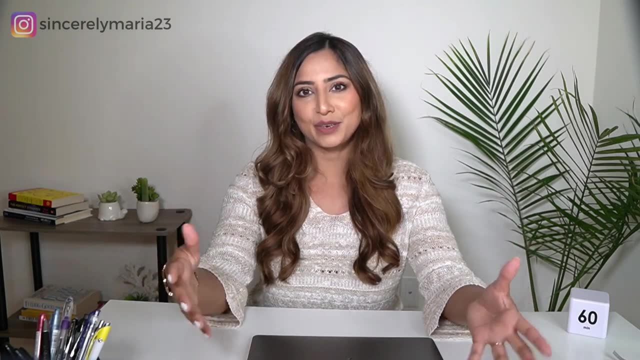 you some time Before we continue to tip four and five, I do want to share a free resource with you, So if you need help on your next presentation or your speech, I have just the thing for you. Grab yourself a free copy of my Public Speaking workbook- Some of the things that you can find. 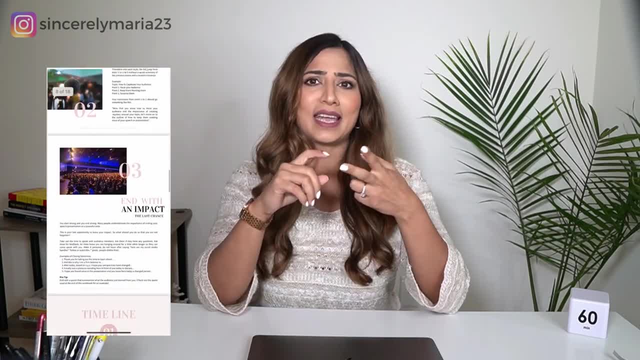 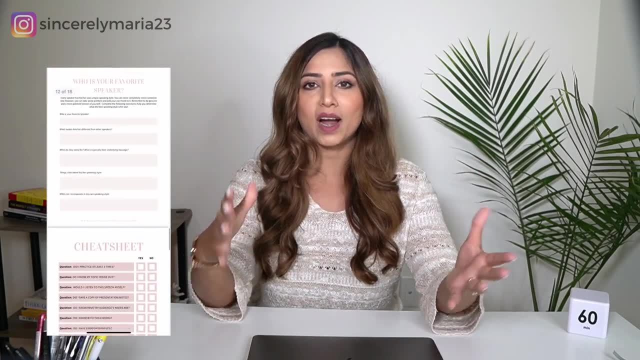 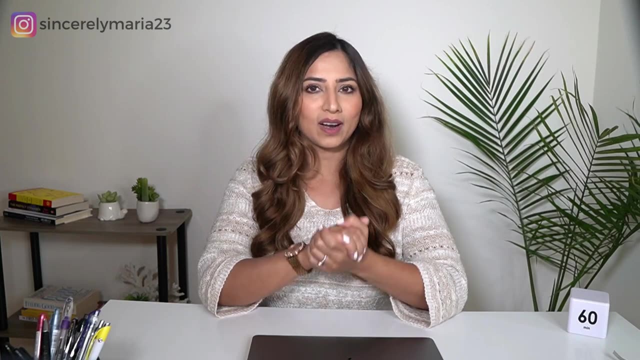 on this workbook are tips and tricks that you can use: a timeline to follow, a goal setting sheet, a story bank, a cheat sheet and so much more. I will leave the link down below, so do get yours today Moving on. So number four of daily public speaking exercises is watch one Ted Talk a day. I am excited about this. Yeah, I am excited. I really am, I'm excited, I'm excited. Yeah, I'm excited, I'm excited, I'm excited, I'm so excited, I'm so excited. So I just want to say thank you so much for that, but I love you, I love you so much, I love you so much. 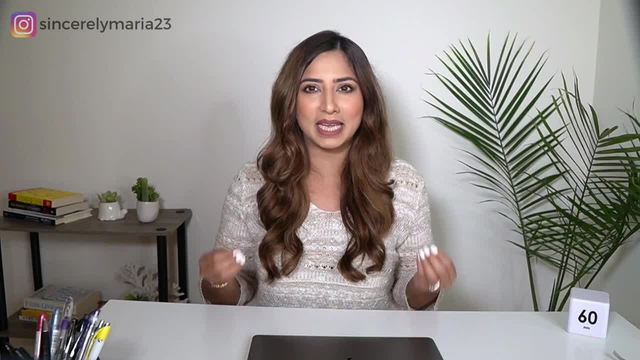 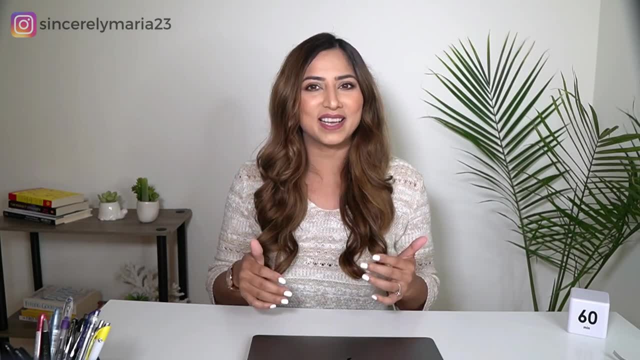 I would love to see you tomorrow. I love you. So listening to this conversation? Sure, go ahead. ted has a youtube channel and there are hundreds of amazing talks from all around the world. these exercises can be just a little bit time consuming, but it also has the most reward. not only are you, 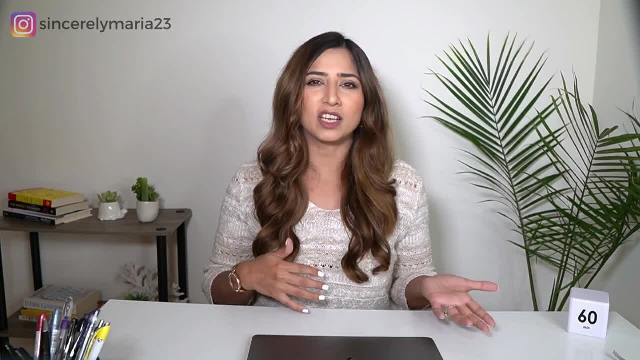 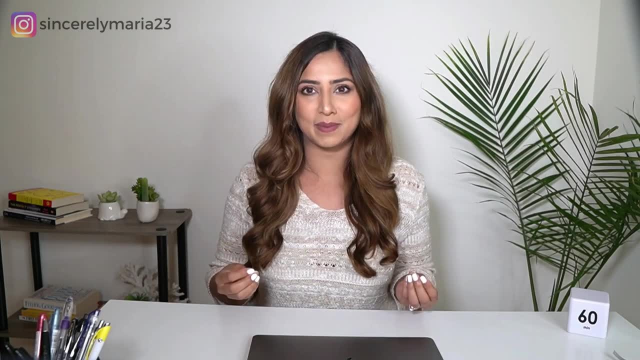 learning about something new by listening to the talks, but by watching the charismatic speakers on ted, you're learning what works well for them and what doesn't. i would pick and choose which speakers you like best and try some of their techniques. watch out for their body language. 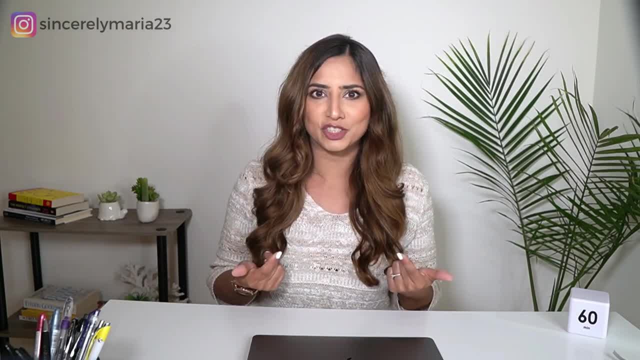 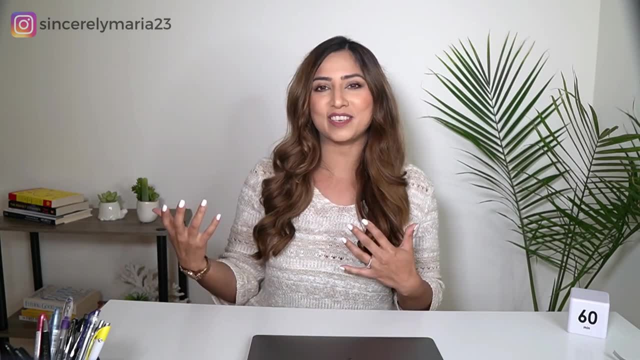 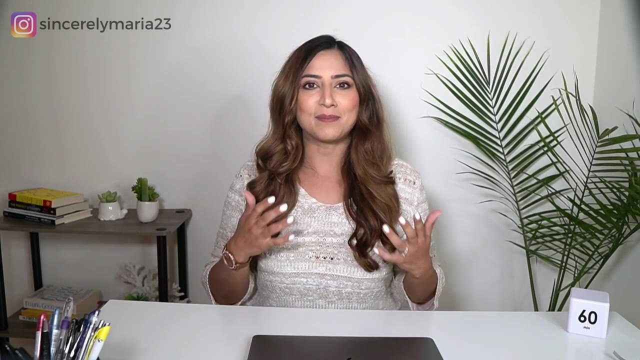 their gestures, their pacing, their facial expressions. try them out for yourself and see what works best when you speak. practice these, especially when you record yourself on instagram, like we talked about earlier, and see what you like and what you don't. once you figure out what you like, start implementing some of the techniques and give your own style and twist to it. so, last, 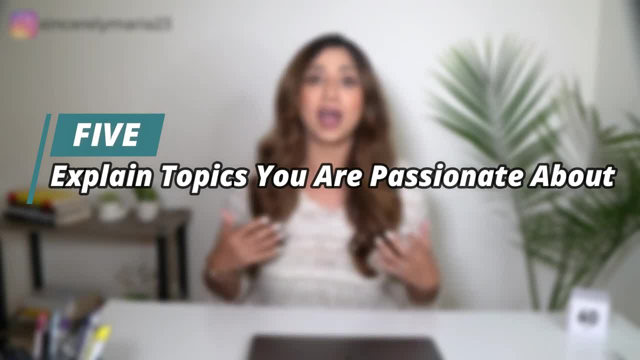 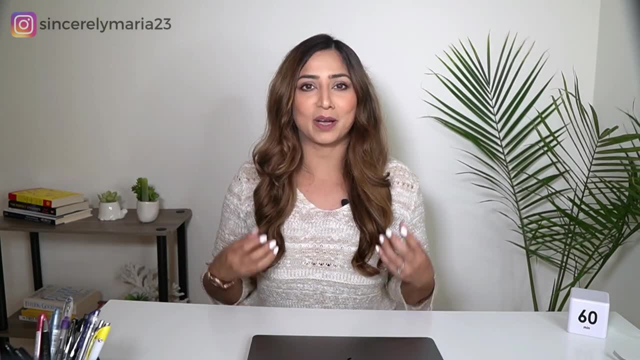 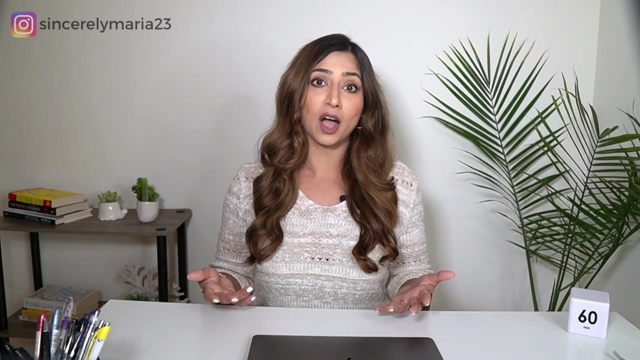 exercise is to explain a topic that you are passionate about to a friend or a colleague. if you want to get better at public speaking, you need to speak to people about your thoughts and your ideas. ask a friend or a co-worker if they have just a few minutes to hear you speak about a certain topic that you think is.